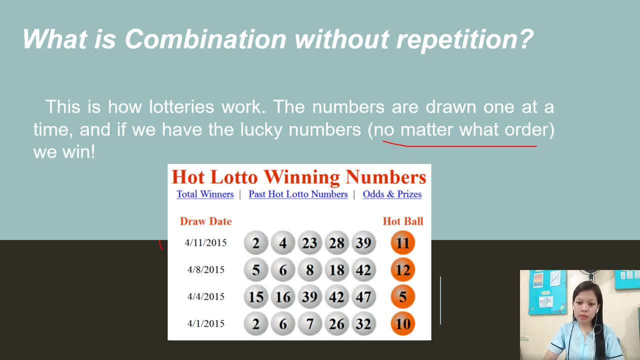 So example for this is the 2,, 4, 23,, 28 and 39. So there is no repetition of numbers. Again, 5, 6,, 8,, 18, 42. There is no repetition of numbers 15, 16,, 39,, 42 and 47. There is no repetition of numbers 2, 6,, 7, 26 and 32.. There is no repetition of numbers. 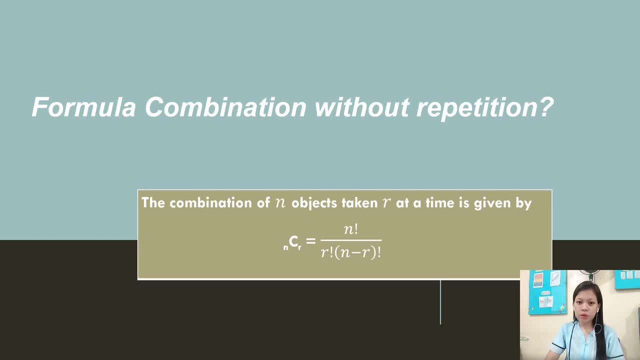 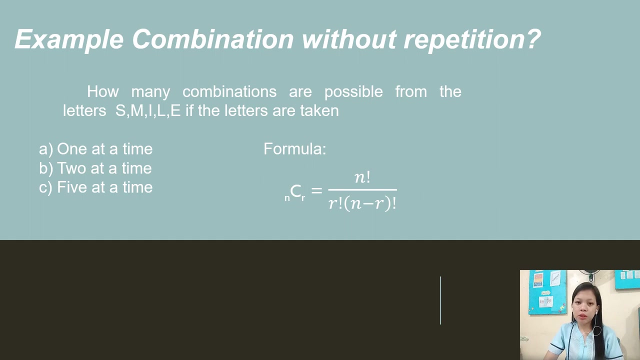 So formula of combination without repetition. So the combination of n objects taken r at a time is given by combination of n objects taken r at a time is equals to n factorial over r factorial times, n minus r factorial. Example: combination without repetition. How many combinations are possible from the last two? 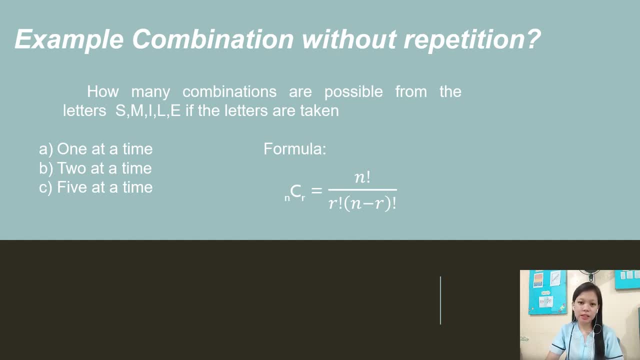 Let's see. Let's see If the letters are taken one at a time, two at a time and five at a time. So we have here the formula: Combination of n objects taken r at a time is equals to n factorial over r factorial times, n minus r factorial. 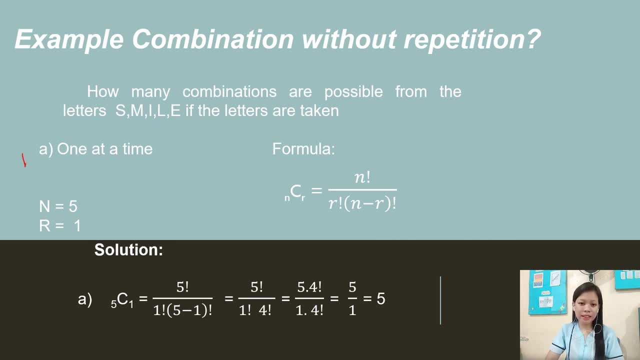 So we have here the example for one at a time. So our n is equals to five, because the word is mile consists. So the formula is this: one Combination of n objects, taken r at a time, is equals to n factorial over r factorial times, n minus r factorial. 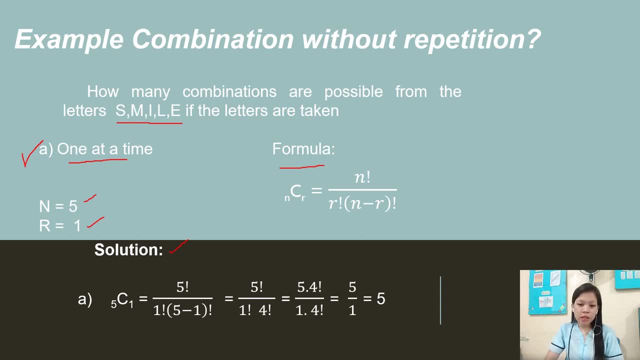 So we have here the solution: Combination of five objects taken r, taken one at a time, is equals to five factorial over one factorial times n minus r factorial. So the answer is five minus one factorial. So substitution of the formula. So we have here five factorial over one factorial, four factorial. 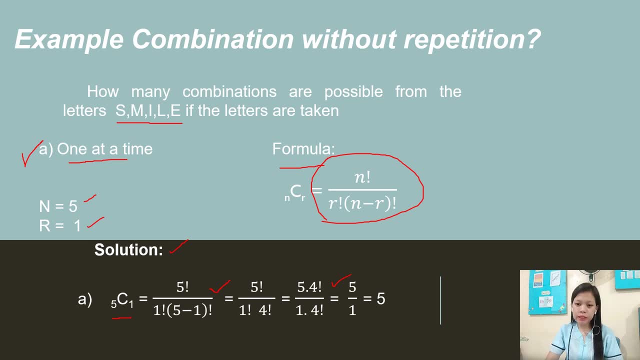 So in simplifying five factorial times four factorial over one times four factorial, So we have to cancel out four factorial And we have here: five over one is equals to five, 5.. So again now 2 at a time. So we have here: the value for n is equal to 5 and the value for r is equal to 2.. By using again the formula, we have here the solution. 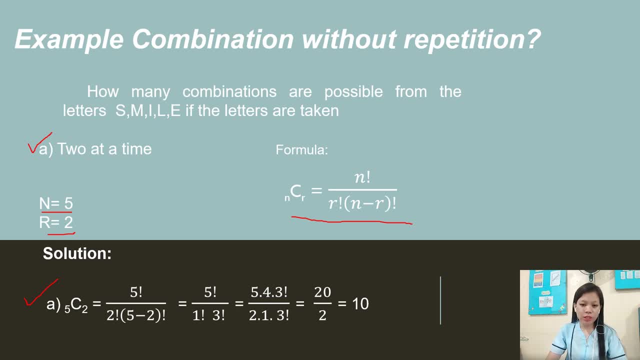 So again, combination of 5 objects, taken 2 at a time, is equal to 5 factorial over 2 factorial times 5 minus 2 factorial is equal to 5 factorial over 1 factorial times 3 factorial. So we have here to simplify: 5 factorial is 5 times 4 times 3 factorial over 2 times 1 times 3 factorial. 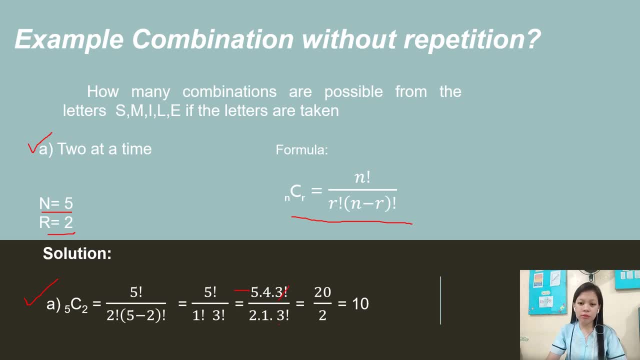 So we have here to cancel out. So we have here to cancel out 3 factorial. So 5 times 4 is equal to 20.. 2 times 1 is equal to 2.. 20 divided by 2 is equal to 10.. 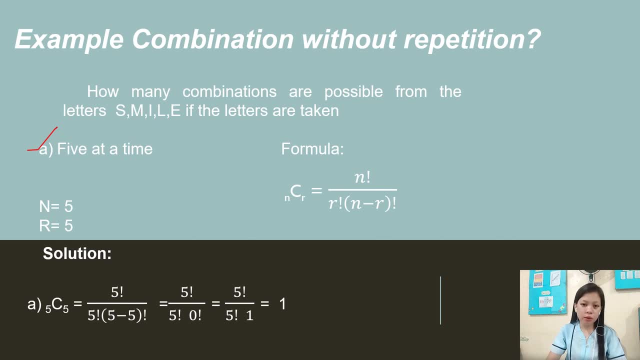 So the example for 3,: 5 at a time. So the value for n is 5, and we have here the value for r is 5.. So we have here the solution: Combination of 5 objects, taken 5 at a time, is equal to: 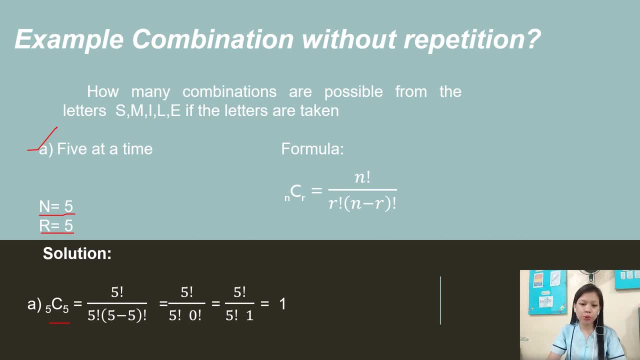 5 factorial over 5 factorial, times 5 minus 5 factorial. So we have here the formula 5 factorial over 5 factorial. So 5 minus 5 is equal to 0 factorial. So there is a rule: When it is 0 factorial it is considered. the answer is 1.. 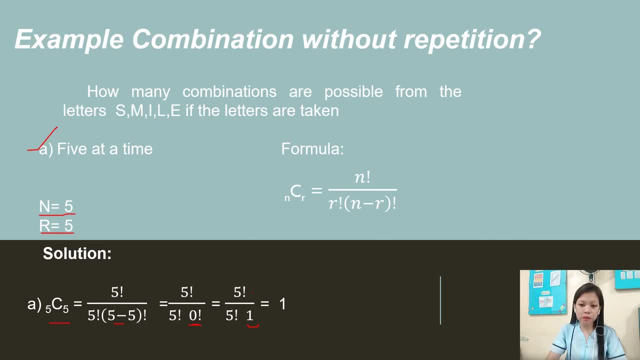 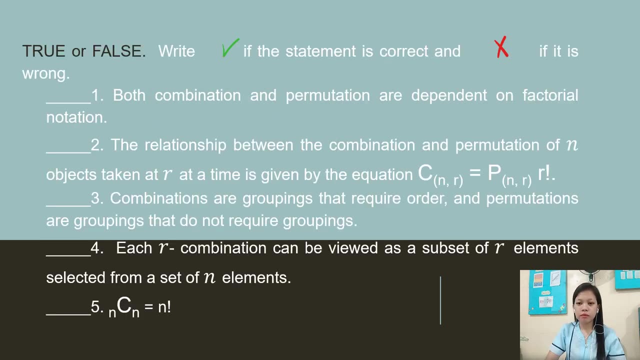 So 5 factorial over 5. 5 factorial we have to cancel out. So the remaining is 1.. So true or false? Write check if the statement is correct. and it is wrong. So both combination and permutation are dependent on factorial notation.